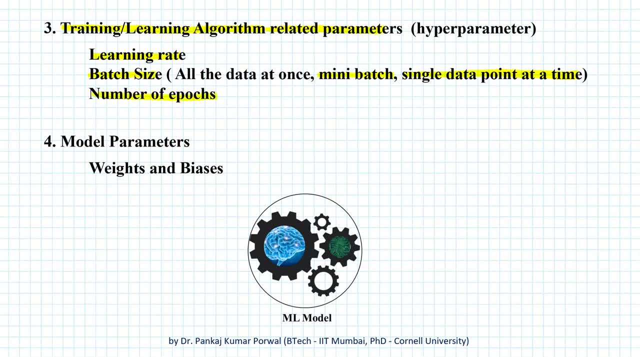 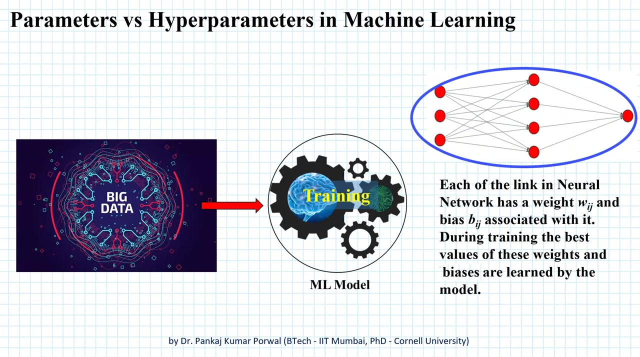 have to decide number of epochs, that is, how many rounds of training we have to perform for our network. once all these parameters are decided, then we come to training. and before the training starts, the model parameters, that is, the weights and biases in our neural network, are assigned random values. for example in: 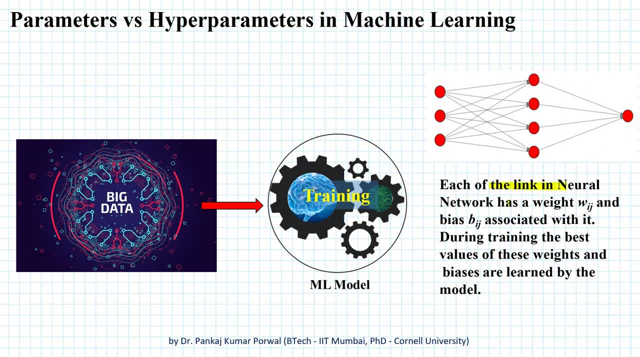 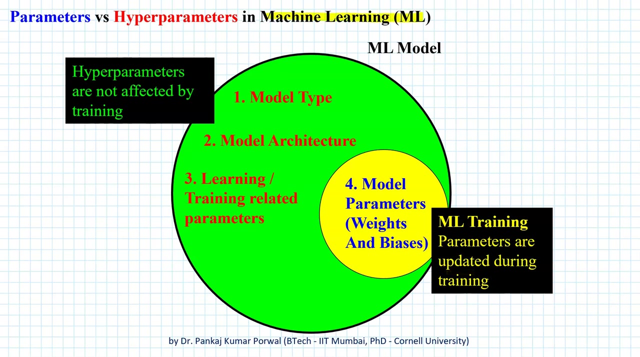 this neural network. each link is a weight and bias associated with it and we assign random values to these weights and biases before the training starts and during training. the best values of these weights and biases are learned by our model. so in our machine learning tasks there are several types of 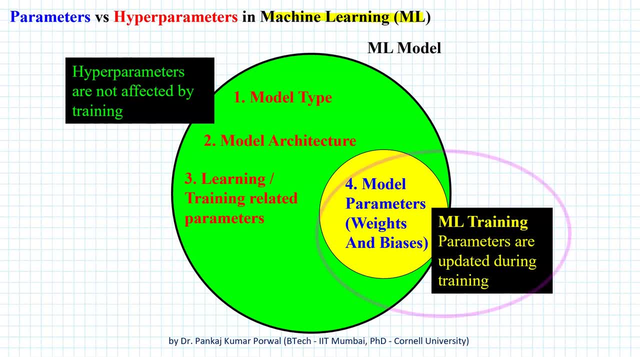 parameters and only few of them are learned during the training, and these are the model parameters and, in the case of neural networks, these are the weights and biases of our links. And all other parameters, like model type, model architecture, learning and training related parameters, are decided before the training starts and these parameters are not. 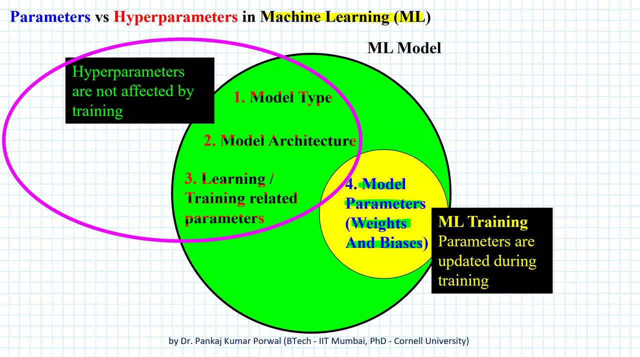 affected by the training. Rather, these parameters affect speed and quality of our training process. So, in a sense, these parameters are over, beyond or above our training process. And if we ask Google, what do we call a thing which is over, beyond or above something? 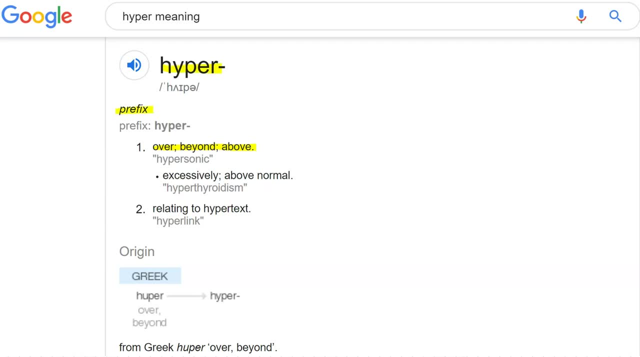 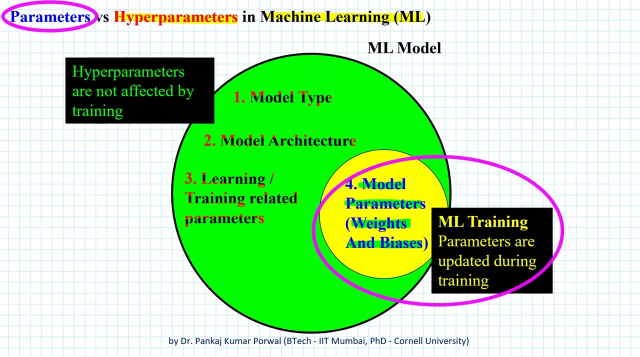 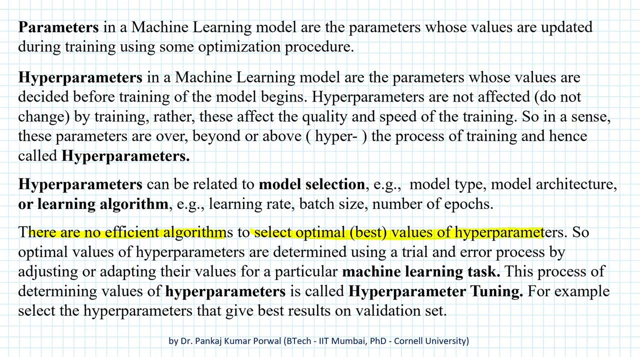 then the prefix for that is hyper, and that is the reason that these parameters are called hyperparameters, and the parameters which are learnt or updated during the training are simply called parameters. So the best values of parameters are determined using training process And, as it turns out, there is no efficient algorithm to select optimal or best values. 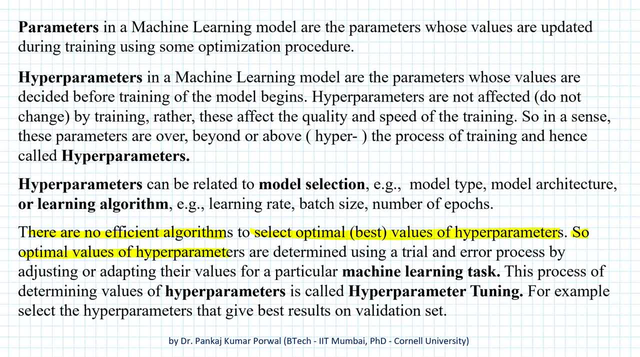 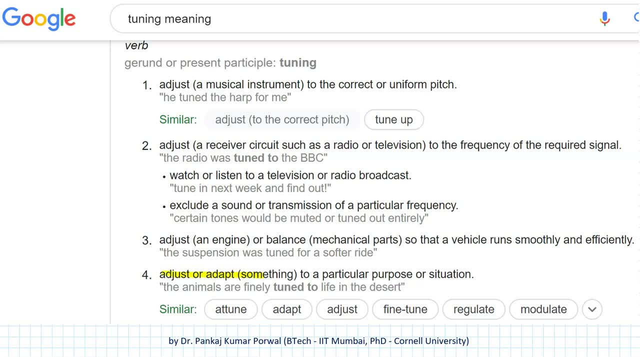 of hyperparameters. So the optimal values of hyperparameters are determined using trial and error process, by adjusting or adapting their values for a particular machine learning task. And if we again ask Google, what is the name for adjusting or adapting something to a particular purpose or situation?